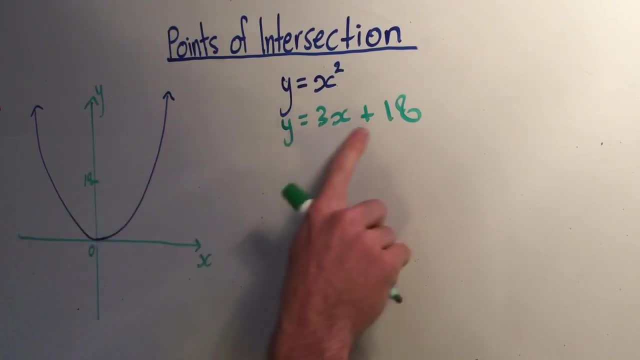 I'm going to make that the y-intercept And it's got a gradient of 3.. So it's quite steep. It's going to be something like that And I'll extend this line so we can see what we're looking at. So let's say it goes there. Now, looking at these two lines together, we can see there's two. 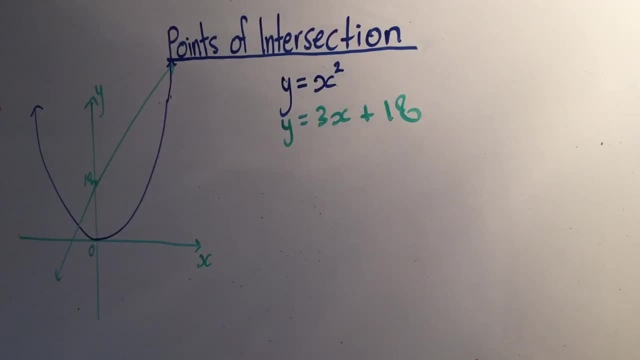 points of interest, And they're called the points of intersection, Points where the two lines intersect or meet each other. They cross over each other at these two points, here and here. What that means is that at this point and at this point, the two lines or 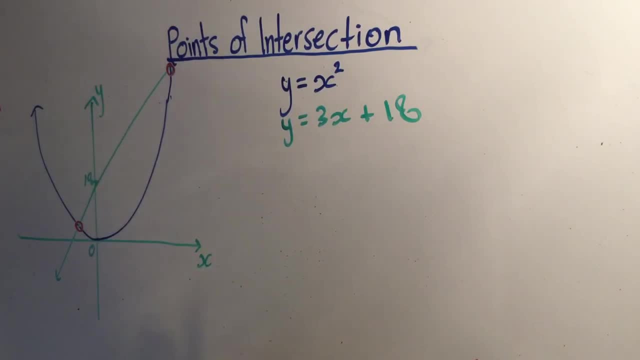 equations have the exact same coordinate, And that means that I could just say that at that point here this y and at this point here this y, The x-coordinate are exactly the same, So they share the same x and y. I'll get rid of that, and 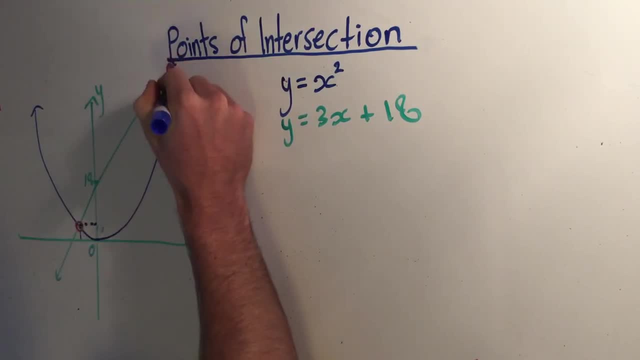 we'll fill it in later with what it is, And also at this one. if we go right down here to the x-coordinate below here, that is the same for both of those lines at this point And I will extend this y-axis for us so we can see where it meets up here. 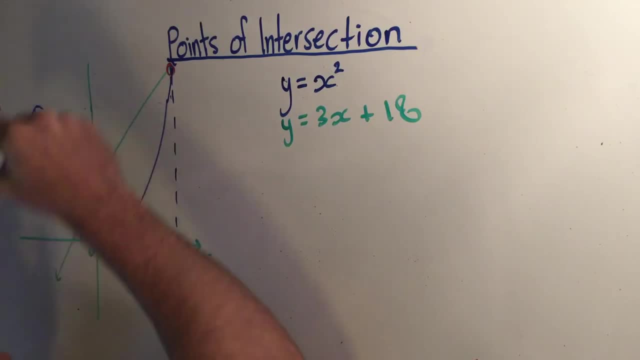 Okay, so that's our y-axis And we have the same y-point there. So the y and the x for this point are the same, and the y and the x are the same for this point, for both of these lines at two points. 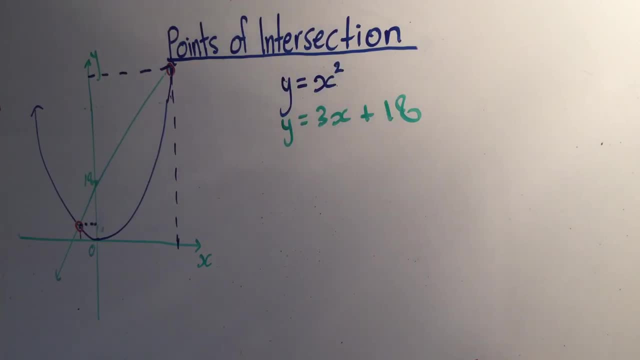 How do we find those two points? Well, think about what we're saying here. We're saying that at this point and at this point, or for any two, if you've got any two equations, you're saying that there's going to be. there may be- we don't know for sure- that there's a point of intersection. 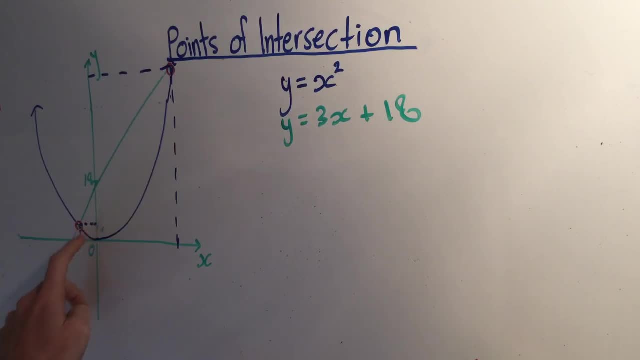 but if there is a point of intersection, we're saying that the y and the x-coordinate are the same. In other words, we're saying at a couple of points here, two points, this y and this y, are the same. So let's make this y the same as this y. 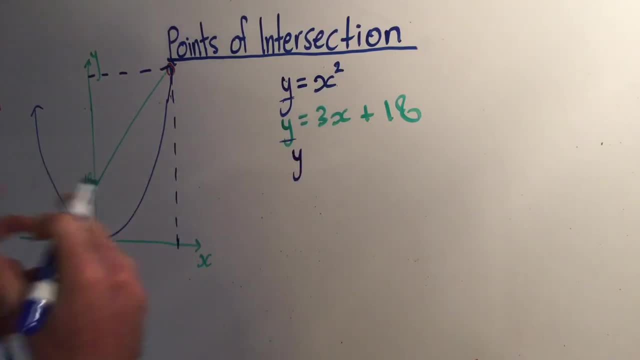 Let's because we know that at the points where they meet, at those specific points, this y-coordinate is the same as this y-coordinate. We can see that that they have the same y-coordinate. In other words, x-squared equals 3x. 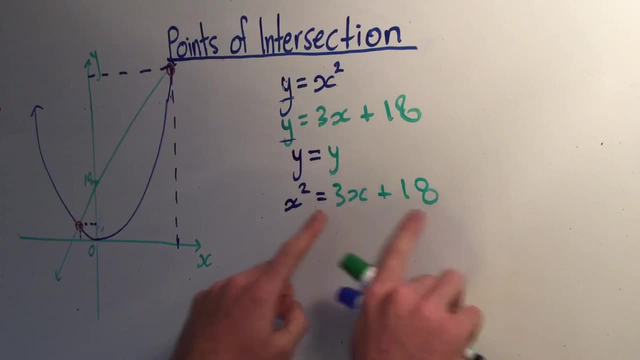 plus 18.. x-squared equals 3x plus 18.. That y equals that y. Another way of looking at what I just did is: I've gone here's this y, which equals x-squared, and I'm going to say that. I'm just going to say that that is exactly the same as. 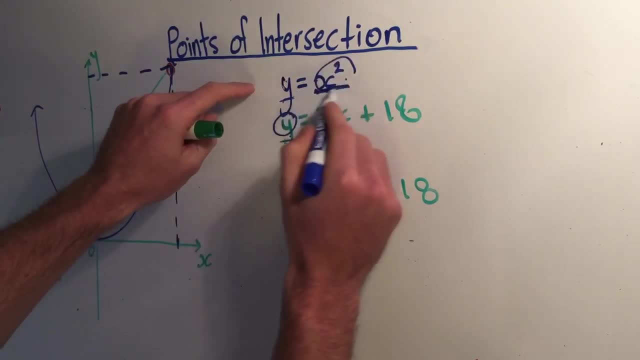 that y. so I'm going to put that in this position because I know that those y's are exactly the same at the points of intersection. Now, when we look at this, we have a quadratic, and when we have a quadratic and we want to solve it, 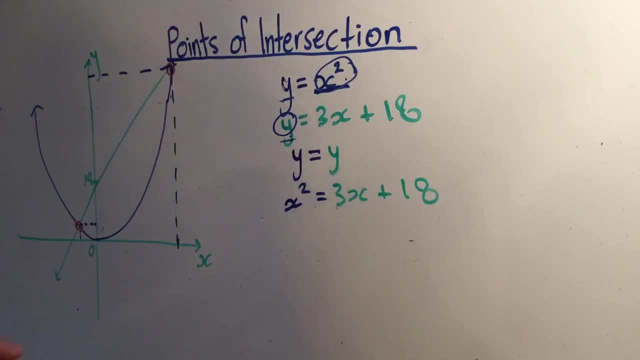 we take everything to one side and we make sure that the side that we take everything to is going to give us a positive x-squared. So I'm going to take 3x over here and 18 over here to the other side. 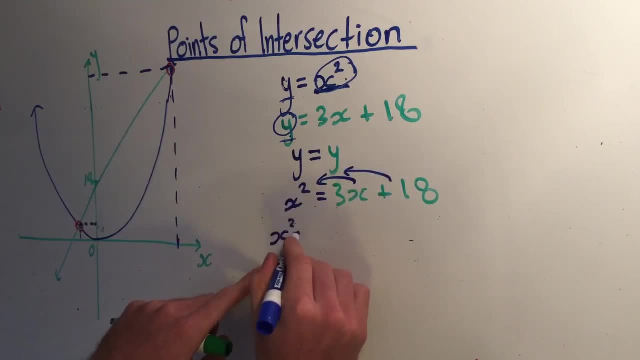 We're going to end up with: x-squared minus 3x minus 18 equals 0.. Now we have a quadratic. Now we know that when we have a quadratic and we're solving it, we are finding the values of x that make this left side equal 0.. 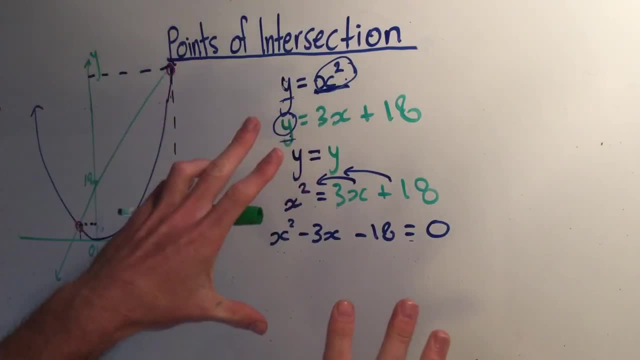 But what does that actually mean in the context of this question? What it means is we're finding the x-coordinates of the points of intersection, because we subbed in where the y-coordinates are the same, therefore, the x-coordinates are also the same. So what you're doing by solving this is you are finding this point and 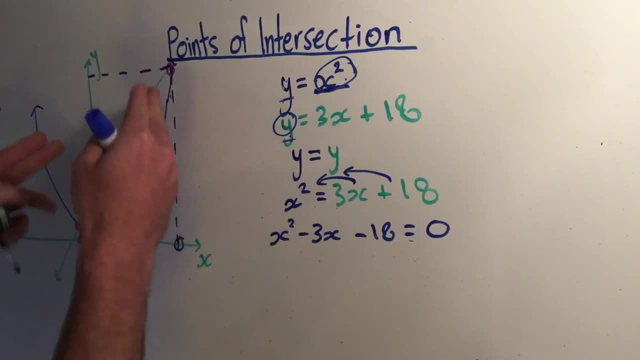 this point on the graph. We're finding what x-coordinate do they have? Because we know these two points have coordinates, We're going to try and fill them in. Right now we're finding the x and that x. Okay, that's what we're doing for that point and that point. Okay, and 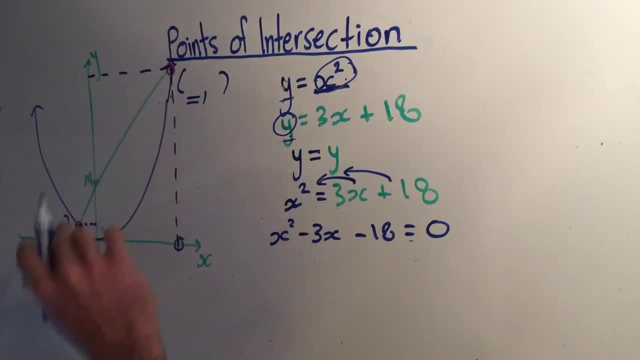 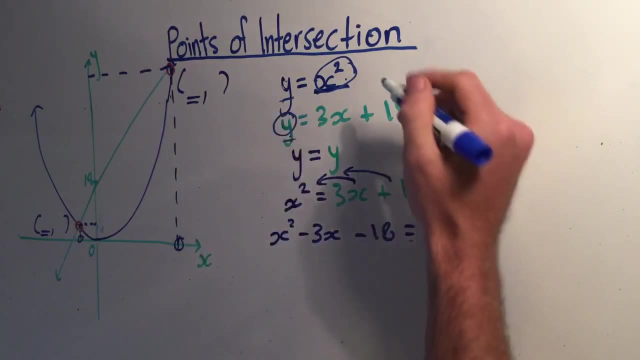 you can do these questions without a graph. I'm just trying to illustrate what we're actually doing. if you were to graph these two equations, So to trace back over quickly what we've done, we got the two equations, we solved them simultaneously. Remember, this was equation number one. 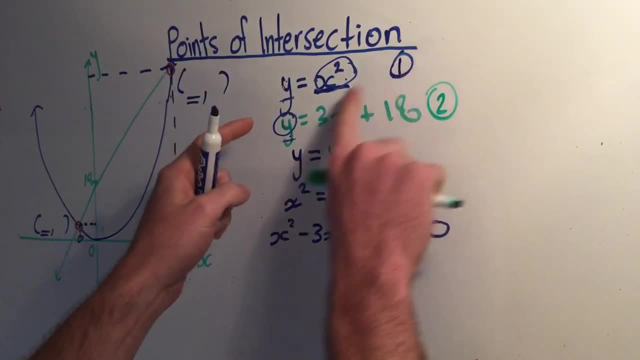 this was equation number two, and we put one into two and we said, or we just made the y's exactly the same. however you want to look at it, Then we've said: x squared equals 3x plus 18, taken everything to one side and now we're going to. 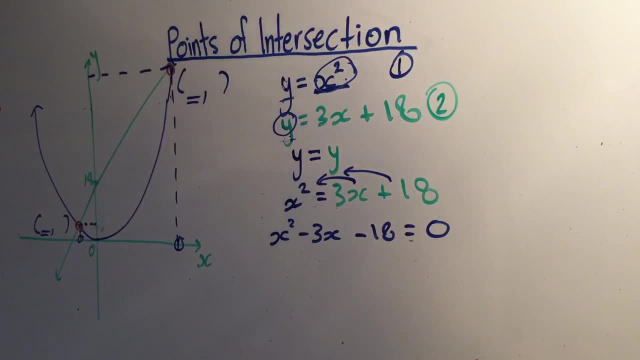 factorize and solve it. You don't have to factorize and solve it. You could solve it straight away. How do you do that? Well, your next step could be to simply use the quadratic form. That's why I have chosen the quadratic formula and sub all the values in to the formula to find the answer for x. 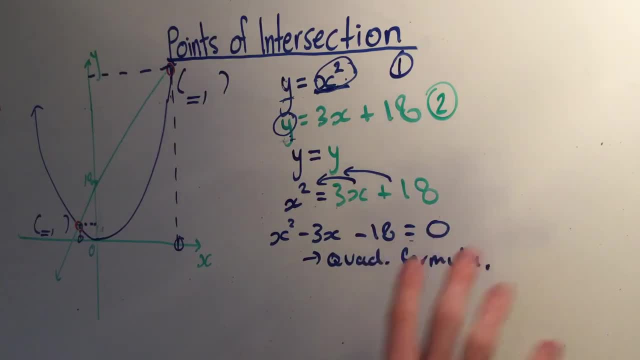 Again, this is only because you've made everything equal, going to be pretty quick and easy if it works. if the psf doesn't work, then you can go and use the quadratic formula anyway. so it's it's a backup method and it's a, it's basically a guarantee to 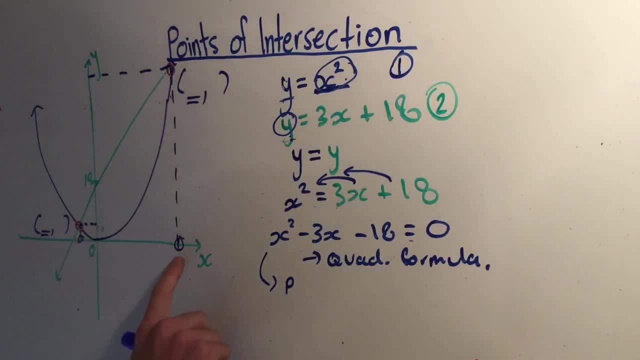 find the answers if there are answers- and here there are going to be some answers, because we can see there are two points of intersection. so, psf, what's our p? well, the p, when we have a quadratic set like this, is the number at the end, including the sign. so that's minus 18. our s is: 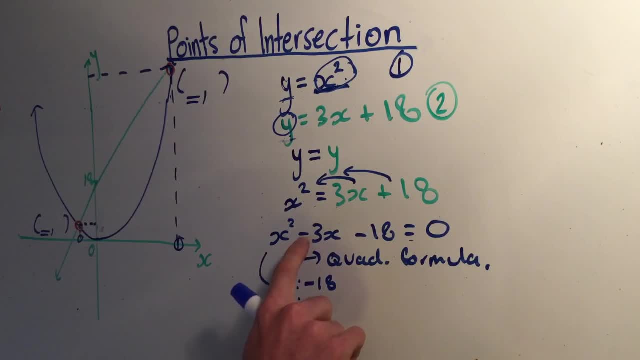 going to be minus 3. it's the number including the sign before the x term. now now i ask myself what two numbers multiply to minus 18 and add or subtract to minus 3? and you always start doing psf by looking at the p first, so let's ignore the s. what two numbers multiply to minus 18? well, i have. 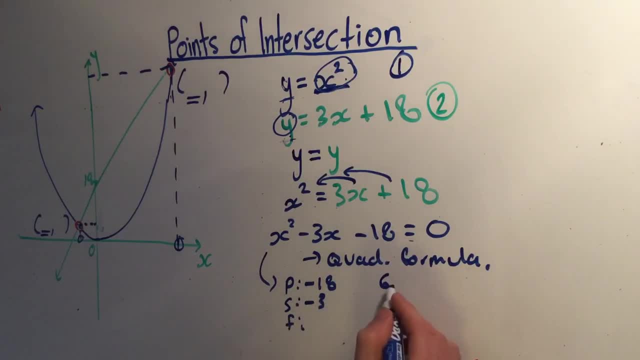 6, 6 and minus 3, 6 times minus 3 equals that, and 6 minus 3 equals 3, that's not negative 3, so that doesn't work. Now I'm going to try the other combination with 6 and 3.. Negative 6 times. 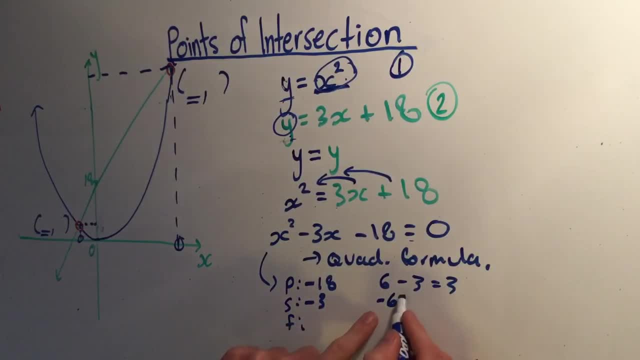 positive 3 is also negative 18, but negative 6 plus 3 equals minus 3, and that's correct. So our two numbers are minus 6 and plus 3.. Make sure you get the signs right. The negative has to be on the 6 and the plus has to be on the. 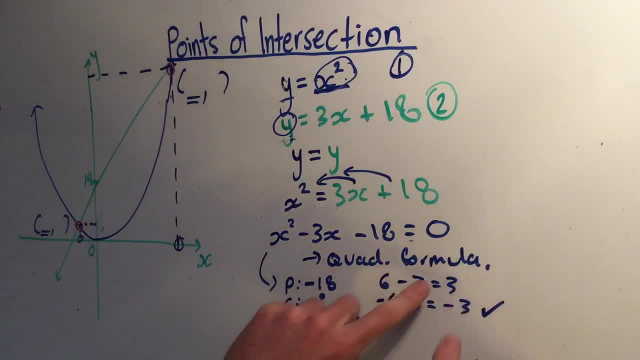 3, for them to add to minus 3.. We don't want the other combination, where you only get positive 3.. Okay, so make sure you try both combinations. Now that we got those two factors, I can rewrite this quadratic and I'm going to rub this out now, So I'll show you how to do that. 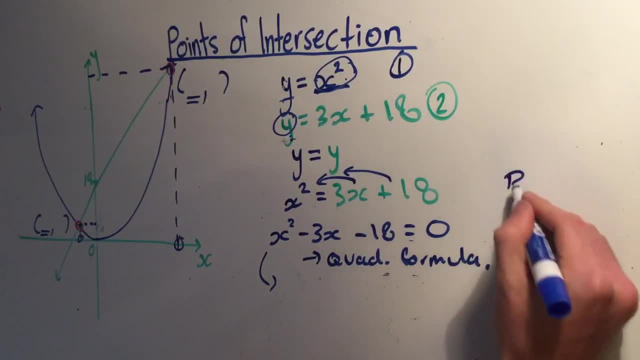 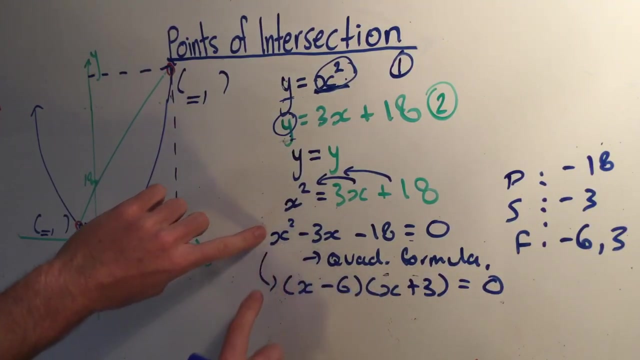 So we figured out up here that the PSF- the two numbers- were minus 6 and plus 3.. So I'm going to rewrite this as x minus 6, x plus 3.. The reason I've put these straight into our brackets with x's is because it is a monic quadratic. That means that there's a 1 before. 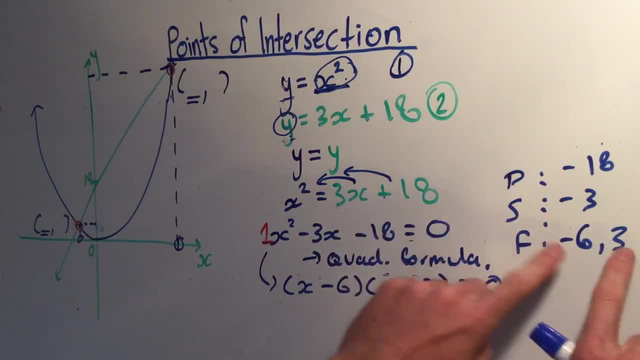 that x squared, which means whatever you're finding is a monic quadratic. So I'm going to put these straight into the brackets next to the x value. You just put x and x there and then you put those. you simply fill these in there and you just have x and x there, because we know that it was. 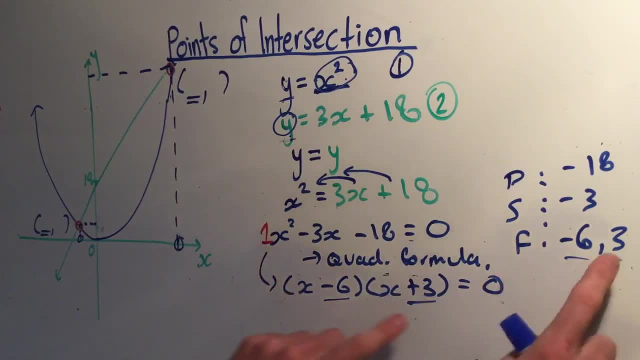 going to be 1: x squared, and x times x is x squared, So you can always pop them straight in. and then how do I make each bracket equal 0? to make the whole left side equal 0?? Well, we can make x minus 6 equals 0, which will give us x equals 6, or we could have that bracket. 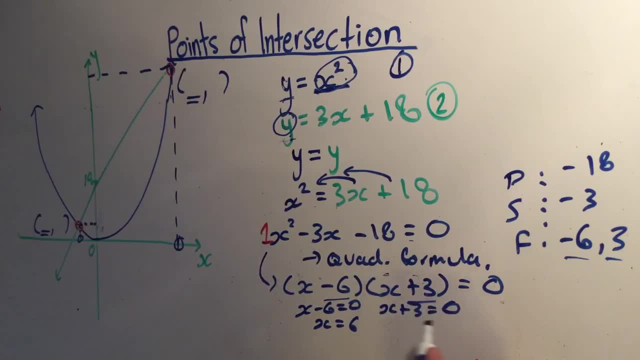 equal 0. So we can make x minus 6 equal 0, which will give us x equals 6, or we could have that bracket equal 0. So we can make x minus 6 equal 0, which is x plus 3 equals 0, and then we take 3 to the other side. 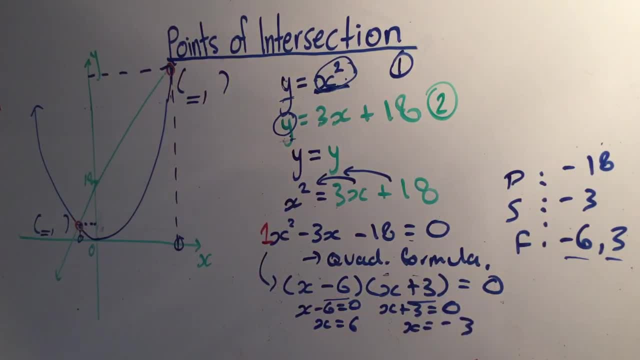 we get x equals minus 3.. Okay, great, what have we just found? We've just found that 6- obviously 6 is talking about this point- is this coordinate: Both of these equations will hit each other at x equals 6, and also they'll hit each other at x equals minus 3, so that point's minus 3.. So you? 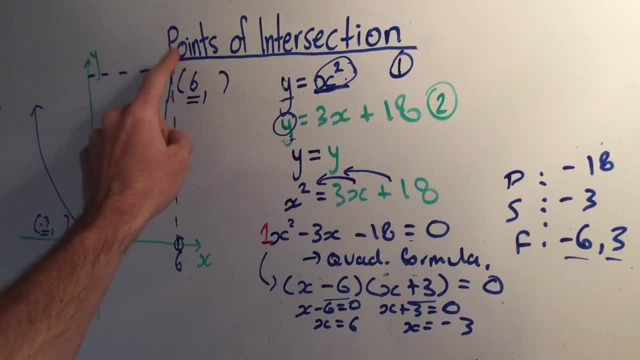 3 and 6 are the x coordinates. let's find the y coordinates because we want the point, not just the x value. So underneath I'm just going to simply write y equals and y equals and remember that we can sub because they're points of intersections and they're the exact same.